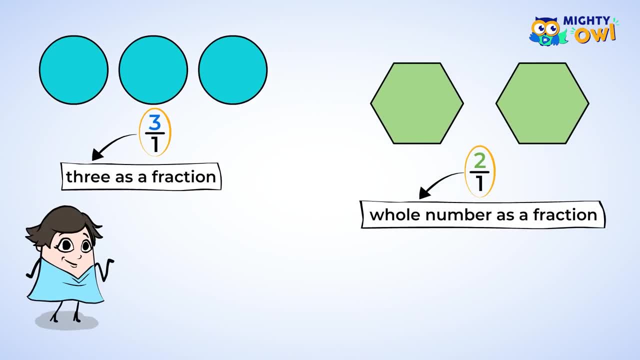 a fraction. Notice that with both of these examples, the whole or regular number is written over one. This is another way we can represent whole numbers. Whole numbers do not have any fractional parts. Let's try this using a number line. Let's try this using. 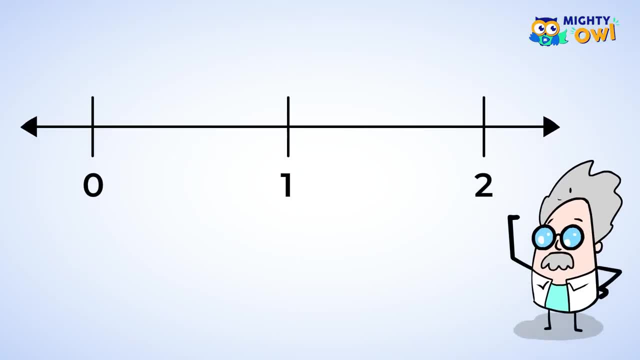 a number line. This is another way we can represent whole numbers. Whole numbers do not have any fractional parts. Let's try this using a number line. We have already looked at splitting the number line up into parts. If we split it into three, 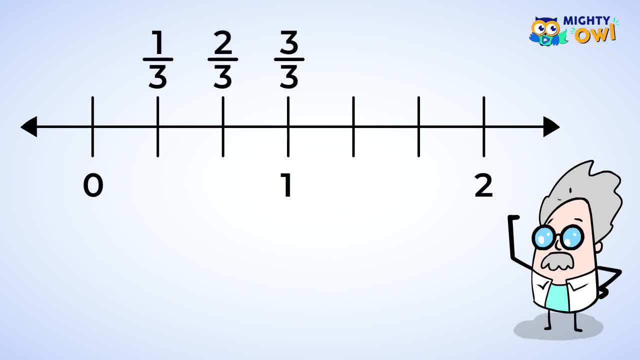 parts. we have one-third, then two-thirds, then three-thirds. Three-thirds is equivalent or equal to one. Do you think we can keep going? Look at that. Six-thirds is equivalent to two, So we can write two as two over one Or as six-thirds. Let's try some practice. 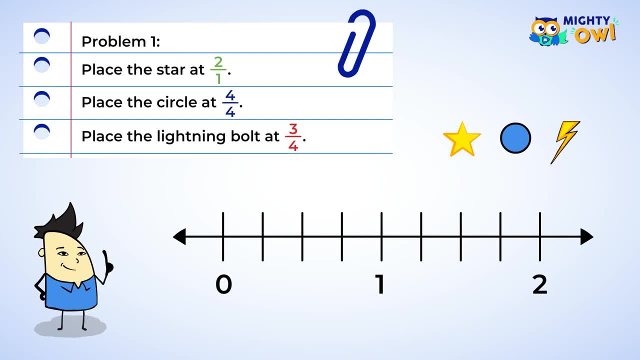 to place these shapes at certain numbers. Let's get started. We need to place the star at 2 over 1. This is the same as 2. Perfect. Next, we need to place the circle at 4 fourths, or 4 over 4.. 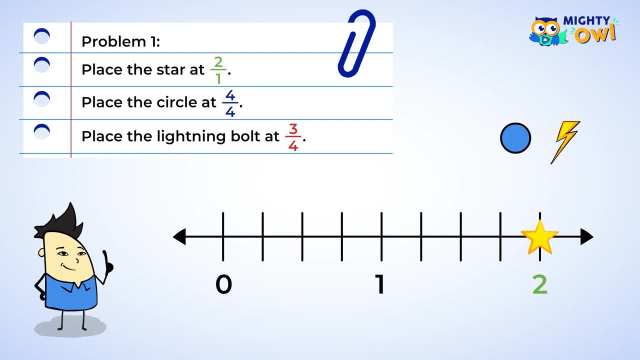 When the numerator and the denominator are the same number, that means you have all the parts of a whole and that is 1.. Alright, last shape, The lightning bolt goes on. 3 fourths. Okay, the number line is split into 4 parts already, which means that starting at 0,, 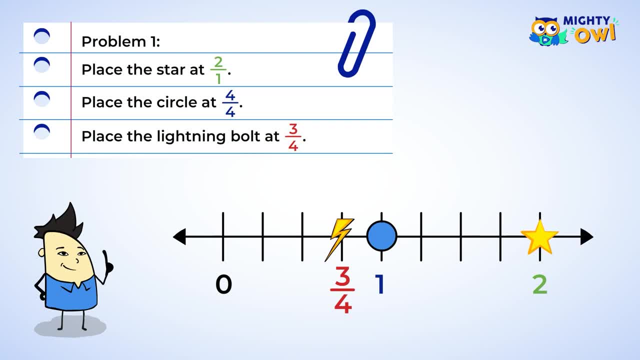 we can count 1,, 2,, 3, and here is 3 fourths. Great job placing all those shapes. Alright, let's try another example. Here we have to figure out which fraction represents point A on the number line. 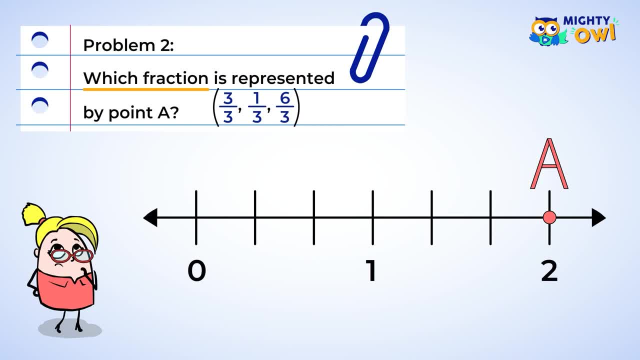 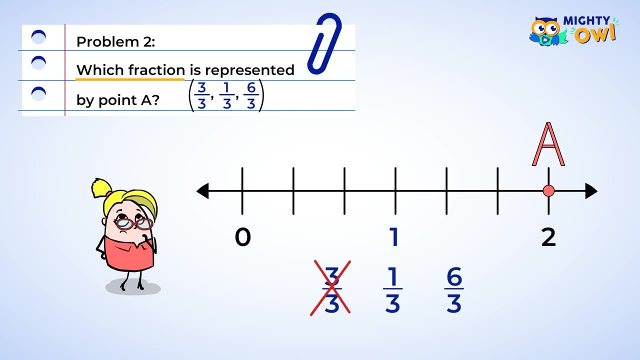 Let's look at what we know about point A. Since it is to the right of 1, it must be more than 1.. Well, looking at our options, we can cross off 3 thirds. The numerator and denominator there are the same, so that's just equal to 1.. 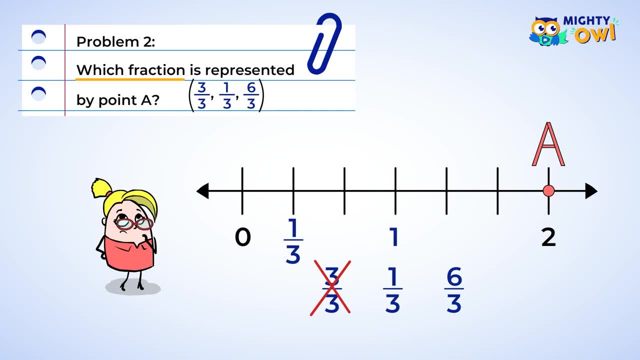 Next we have 1 third. This fraction means that only 1 section out of 3 are shaded. If it were a box, the whole box wouldn't be shaded. That is less than 1 whole. Our next option is 6..